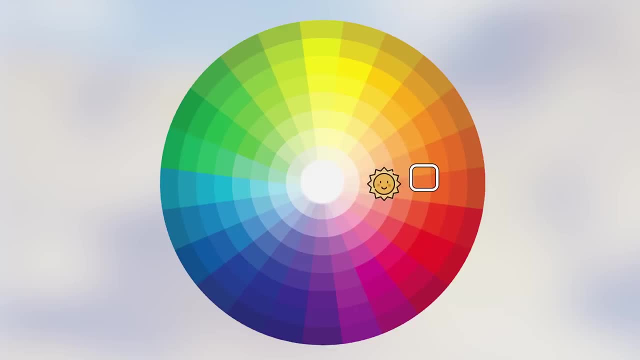 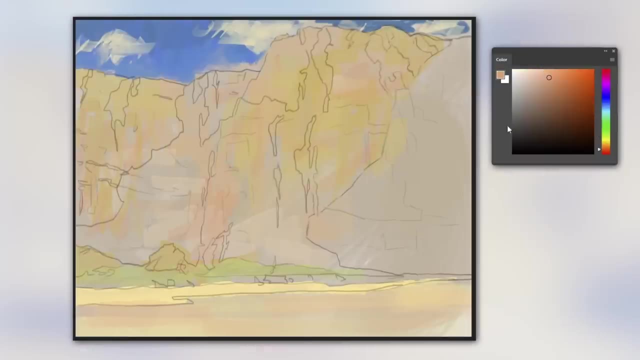 Saturated sunlight adds saturation. So where that color swatch is now, we could use that to represent sunlight on the rocks At that time of day. okay, but you might notice that my rock colors have some variety to them. That's a bit of an extra. 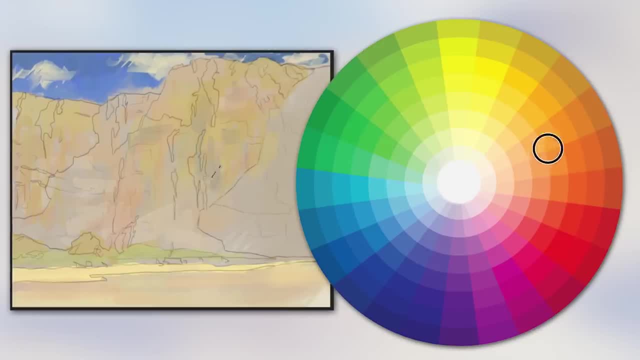 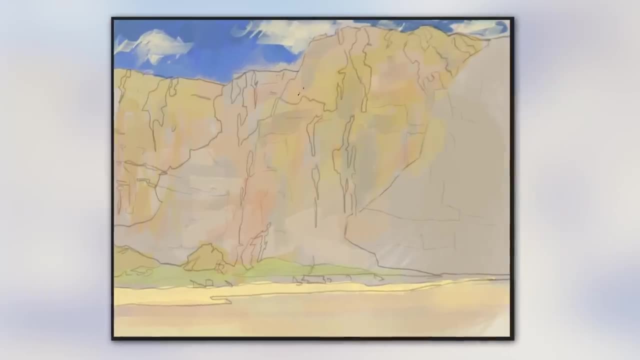 artistic layer. I'm taking that color from where we calculated and just wiggling it around. The amount of wiggle is up to you And it can be a negotiation between the reference and what you want your art to look like. Alright, getting back to 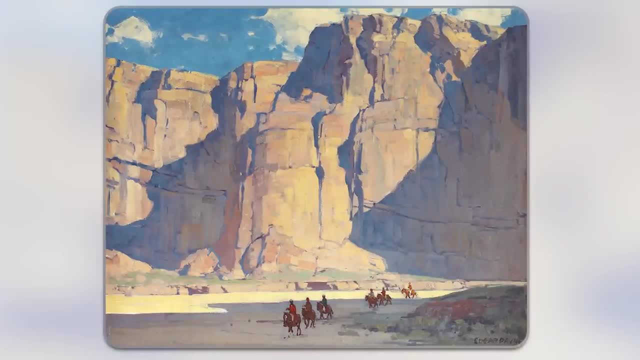 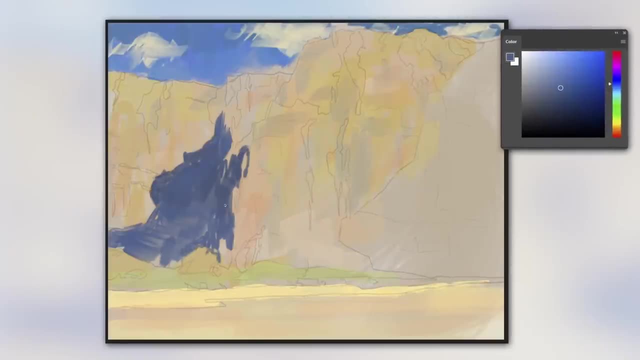 the reference here. it's time to put in those shadows Now. there is so much beautiful color in those shadows which I'm going to ignore at first. I'm painting with basically one color Here and one value. I'm mostly focused on the shapes. I'm choosing a blue color because we're outdoors on a sunny day. 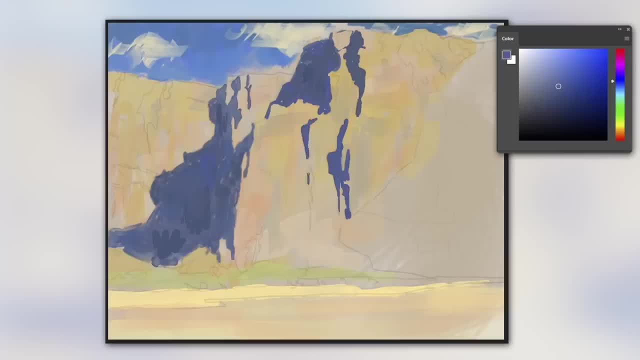 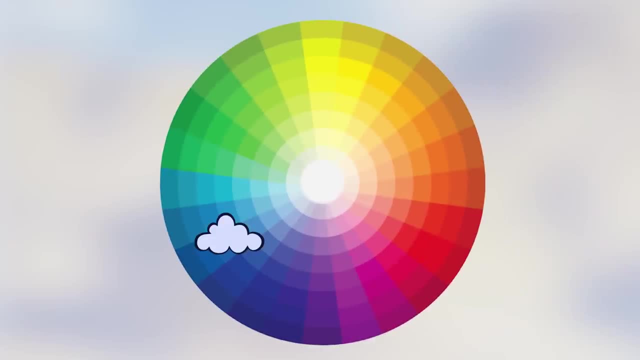 there's a big blue sky up there, casting lots of blue ambient light down into the scene, which we can perceive in the shadows. I'll show you how this works. The sky And this painting is pretty saturated And the base color of our rocks was here. 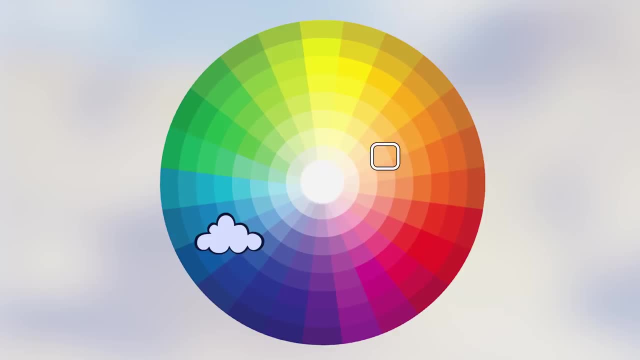 That's the base color of the rocks, without the sunlight. Now Remember when I said that, neutral the sunlight would not pull the color toward it. That's because, the sunlight being neutral, there didn't have a discernible hue, let alone any saturation. Back here now. 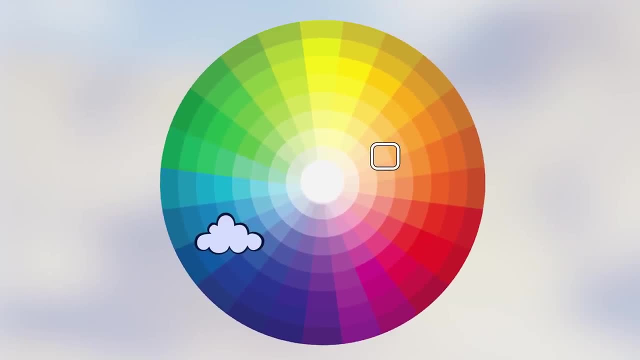 this is a very saturated blue light and because we're talking about shadows, where there is no influence of direct sunlight, the saturation will be strong enough to pull that color right toward it. Where you stop is again up to you. I could stop about 80% of the way, which I think is about. 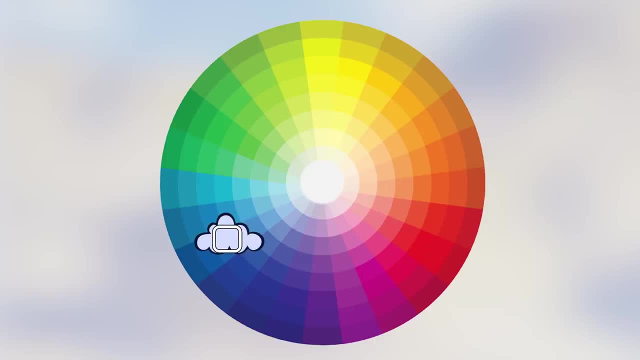 how nature would do it. or you could go all the way And you could wiggle it from here too, but when I do, I'm more or less going to keep it in one hue. for now, That leaves a saturation wiggle which looks like this: So back in the painting. it's just that simple. This is basically. 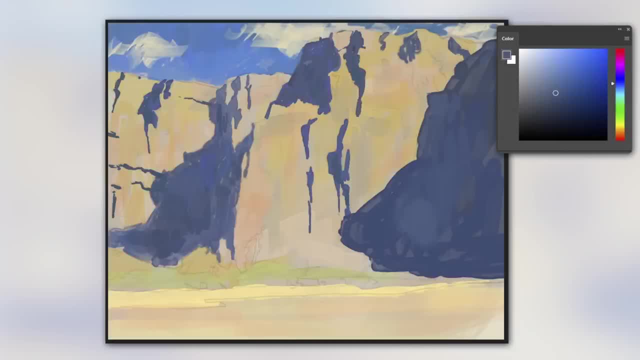 a two-value painting, despite the color varieties. The simplicity is a chess move. I'm setting the stage for a color attack later, And that's where the heart of this study really is: the color in the shadows. Here in Blender, I've mocked up a scene to show you how shadow colors outdoors. 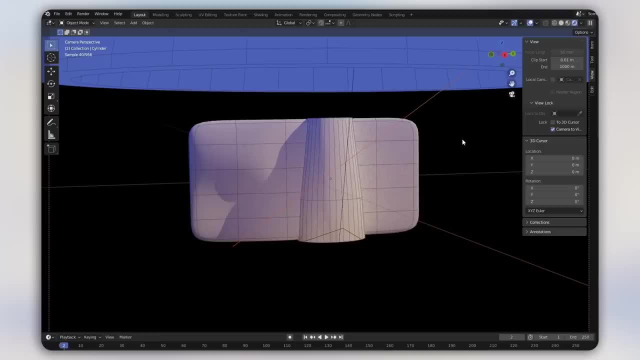 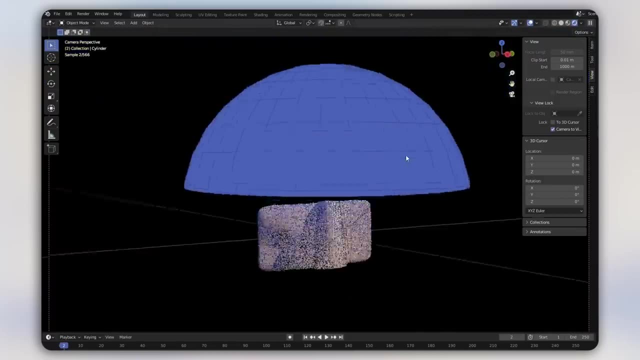 typically work. This line here is the direction of the shadow, The direction of the sunlight. Then, typically, that sunlight hits the ground and bounces up. represented by this light, The blue bowl of the sky is huge, of course, and casts blue light. 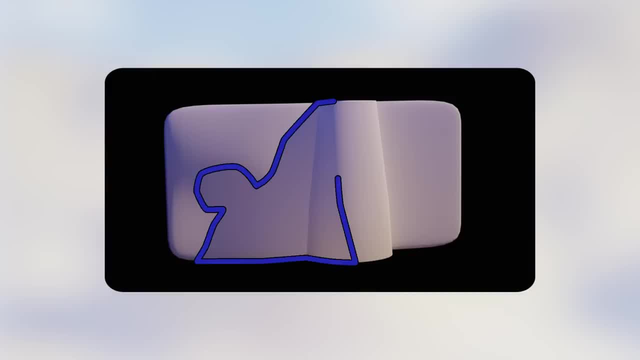 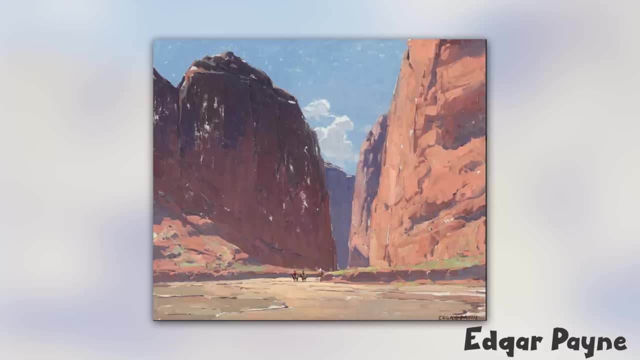 downwards. So what we typically see inside our shadow shape is a color transition from warmer at the bottom to cooler at the top. Here's another painting by Edgar Payne where you can see this clearly. The sun is up here casting light down, and its bounced light influences the bottom part. 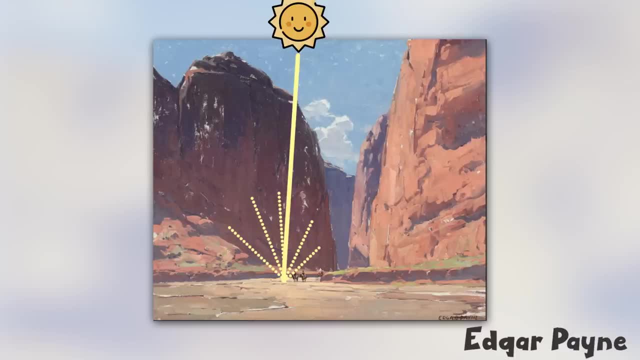 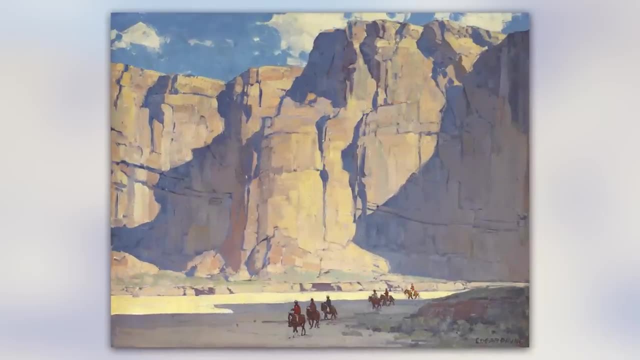 of the cliff, Because that's the area that's most important to us And that's where we're most available to it, And the blue skylight is, just the same, showing up most at the top, which is the area most available to it. Now, plot twist, this painting doesn't do that at all. This color. 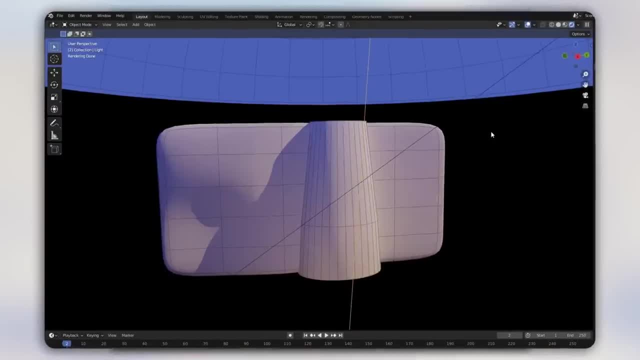 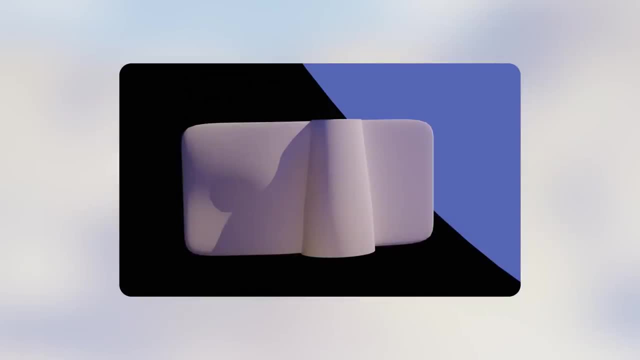 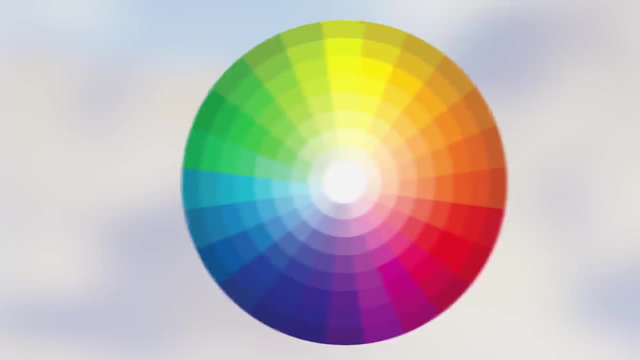 transition goes from left to right. It's almost like Edgar Payne decided to play God here and rotate the sky like this. In this configuration we do get that left to right transition. So I didn't see Edgar Payne's reference, but I'd wager it was a design choice he made there To pull this. 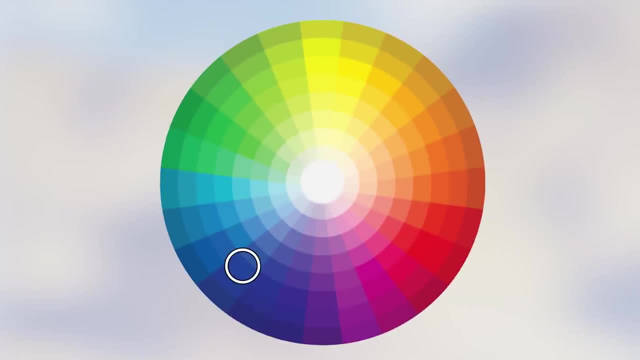 off. we have to go back to the beginning of the painting. We have to go back to the beginning of the painting. We have to start from our current shadow color and then decide what's the warmest we want to get. I'm going to put the warmest shadow here, which is generally less saturated than most. 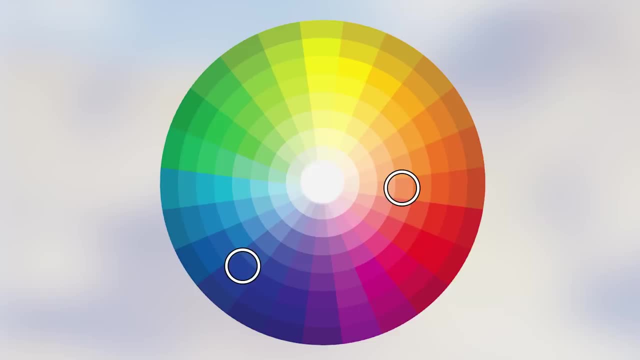 of our lights were. Next, we got to figure out the path we're going to take to bridge these two colors. This is generally the wrong path. There's just nothing to motivate those saturated purples. You could just do a straight line between the two colors and this would work. Nature, however. 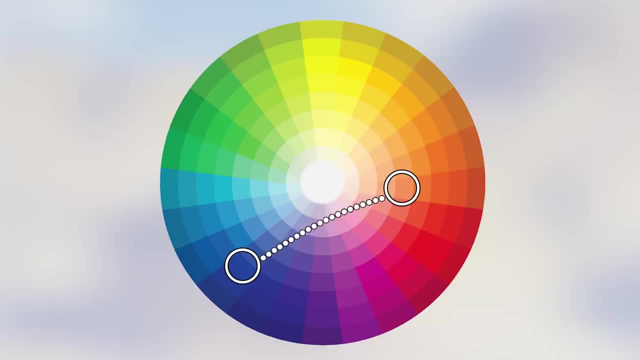 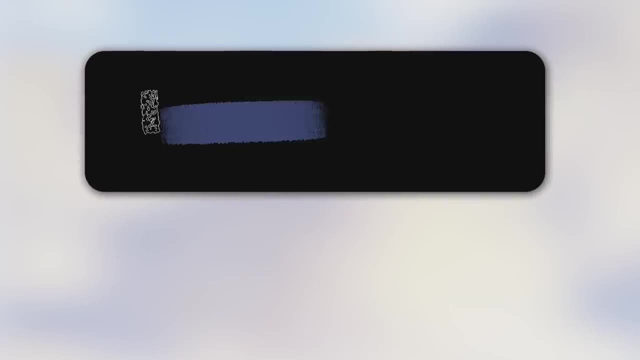 treats gray like a gravity well and it'll pull the color towards the center of the painting. It'll pull the color towards the center of the painting, especially when crossing through it. That's the path Edgar Payne is using. It's helpful to do a little practice run. Take a swatch of base. 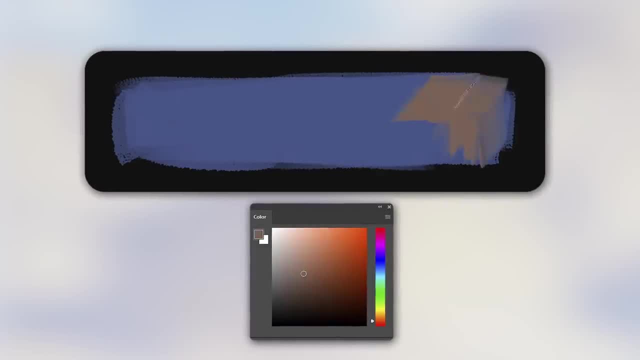 shadow color. then go ahead and find your warmest shadow color. I'll mix it in there with a smudge tool. Now, using the path we just plotted earlier, try and make the first step from the blue base color to the resulting warm color. It may look odd at first. After all, we are warming a blue here. 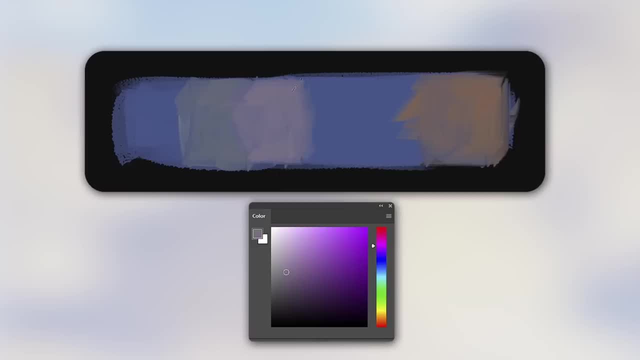 That's a bit weird. You're playing with the grays and subtle hue shifts Step-by-step. plot points on the path. Put swatches down. I really recommend using soft edges when transitioning subtle colors like this. That's why I'm using a smudgy tool. Anyway, see if you can. 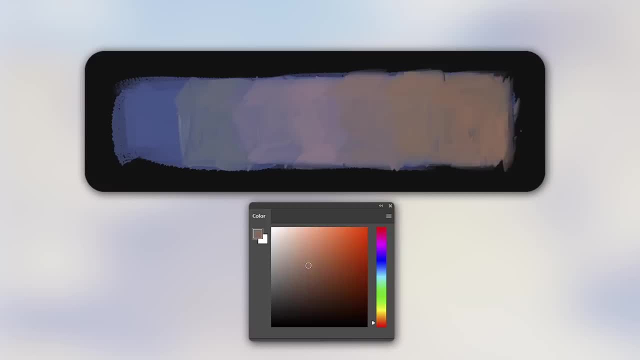 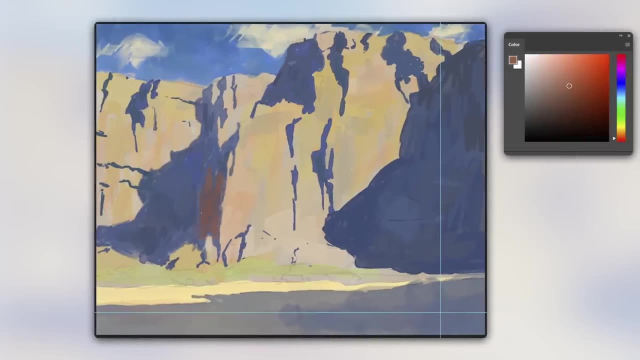 come up with between four and six colors that smoothly show the transition. All right, so let's actually paint this. I'm going to start with the warmest color in the shadow. Notice on my color picker: I've overshot the color. It's too saturated, But the smudge tool helps me blend it into the. 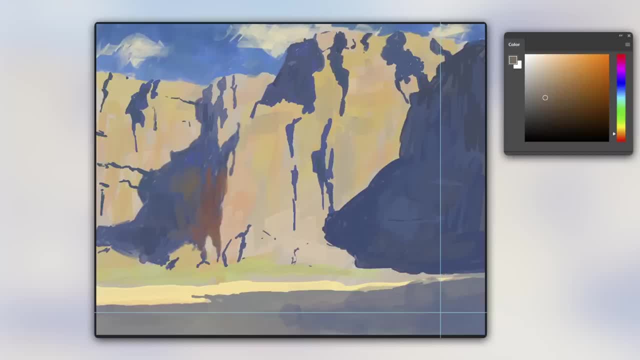 blues, just the way you would mix oils or acrylics. At this point, I'm going to go ahead and paint the shadows. At this point, these warms in the shadow may look like they're competing with the light's warmth, But if you squint your eyes, look at how it all melts back into blue. This is largely because 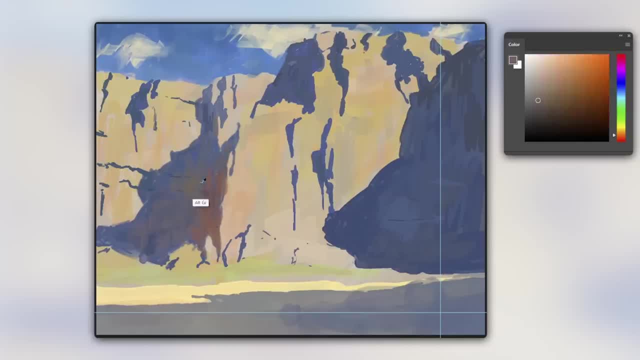 the value is not changing very much. What I'm painting here is reflected light. Reflected light bouncing up or to the side, as we've established, from the ground. So, being reflected light, the value will get a hair lighter than my base shadow value, But it's half a hair, almost nothing, See. 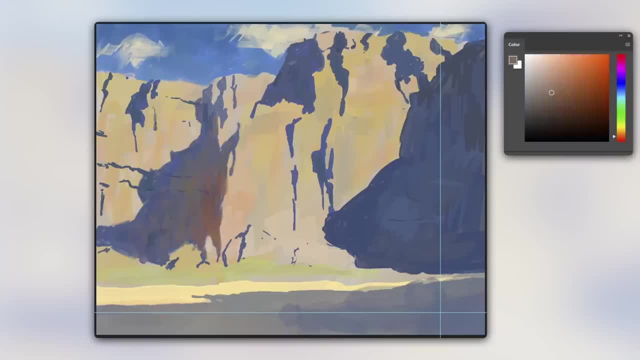 if you use too many disparate values in the shadow, you're going to end up with a shadow that's not in any given area. You'll end up over-modeling the thing And that just torpedoes any effort you put into the color. That's because value is more fundamental than color, at least in this style. 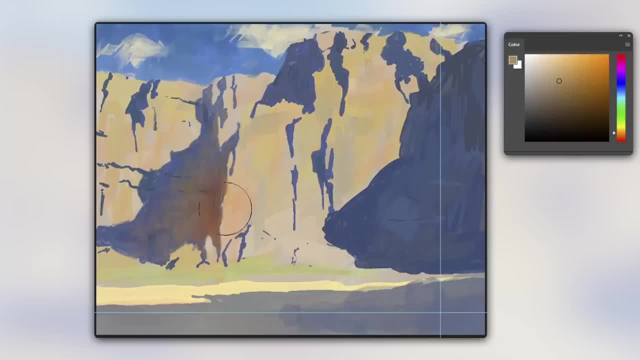 of painting, And here I've got an overlay airbrush just punching things up where needed. Speaking of airbrush, you could approach it this way: Look at this shadow. I'll use an airbrush set to overlay, to put in that warm tone, And I'll use those airbrush-y soft edges to my advantage. It's. 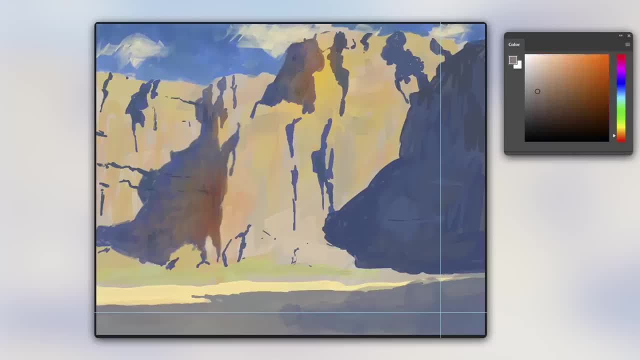 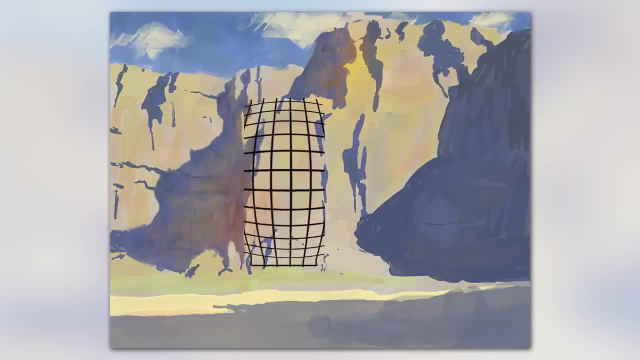 maybe a bit more natural to work into those soft edges with any kind of smudge mudgy tool. Alright, so it's coming along, everything is in control, But some of these cliff faces are flat and they need a bit more form. This area is essentially cylindrical, So 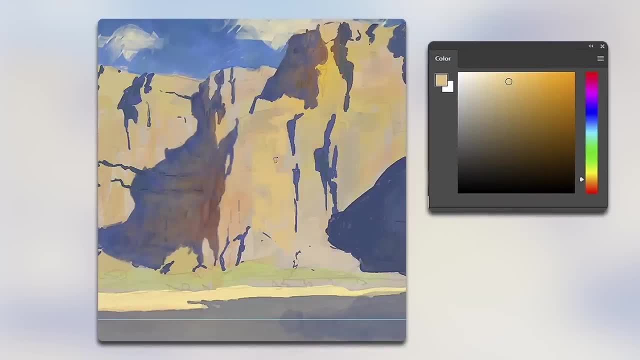 here's how I'm thinking about the color In the parts of that cylinder that face the sun more directly that I'm painting right now. I will increase the value of the yellow-orange color Because, as we established at the beginning, that is the color of the sun at this time of day. 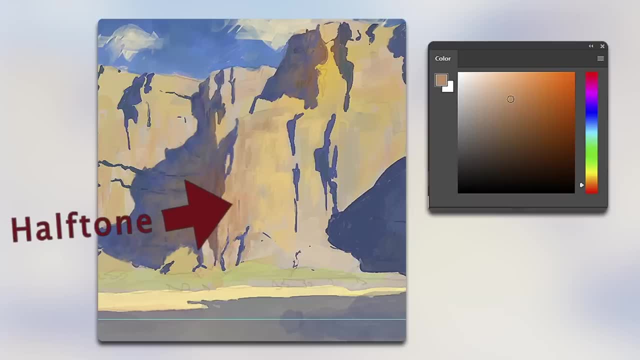 Now here I'm putting in what's called halftone. Halftone is difficult. It's a color and value that live in the light family, But it's gotta be a bit darker than the average light in order to turn that form. It can be confusing to figure out which color to use. 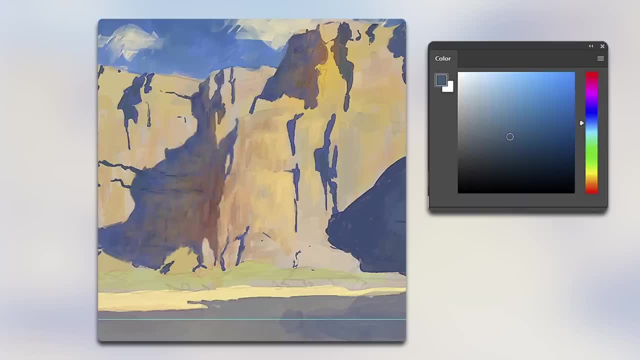 for halftone. After all, it can't be blue because that's the realm of the shadow, And halftone is not shadow, But it also should probably not be the same color as the stuff that gets directly hit by the sun. So here's how I usually think about it. 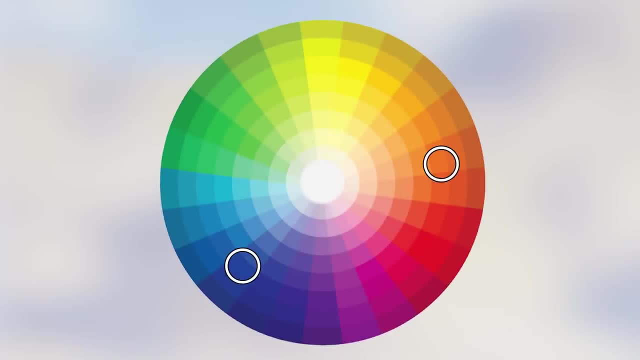 Our sunlight color is around here And our blue shadow is here. This is the path I plotted before The gray gravity. well thing. So because halftone is still in the light, you could move your color about here. Something remaining in the realm of the warms. 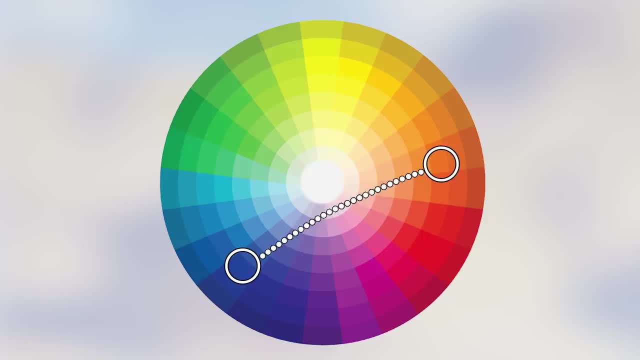 And this would work. However, with halftone, you don't necessarily have to observe the gray gravity. well, You can do the thing I said you shouldn't do when going from light to shadow This path, Because, remember, the path ends about here. The gray doesn't have a chance. 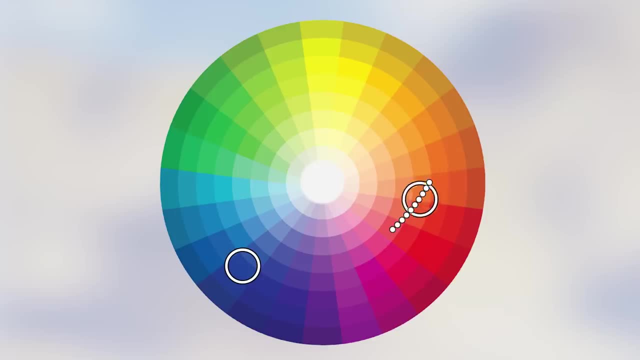 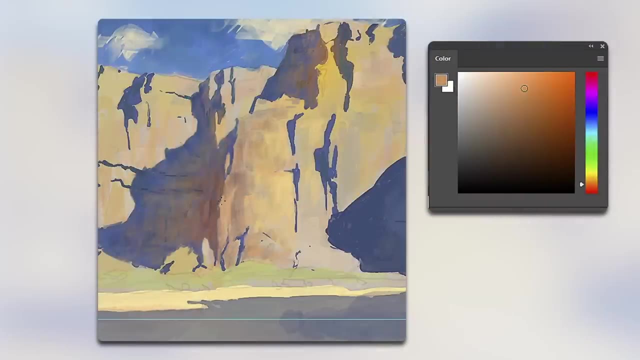 to exert its gravitational pull, So you can do a move like this. That is a more reddish color As opposed to the yellow orange, And you can keep it fairly saturated. So while I'm painting this halftone, I'm actually using both of those paths. 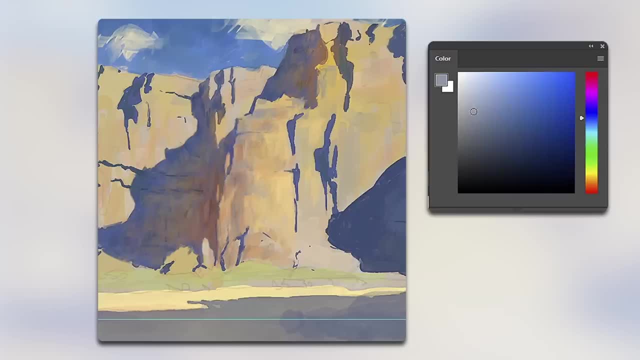 The path that observes the gray And the path that uses more saturated reds. I'm using soft edges to mix one into the other. Again, they share one value, so it's okay to do that, And I'm just distributing those colors with my own visual aesthetics. 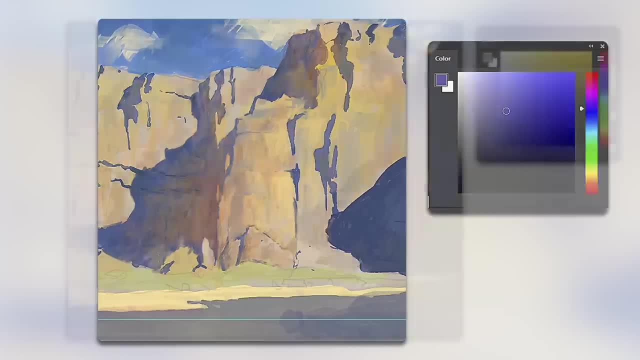 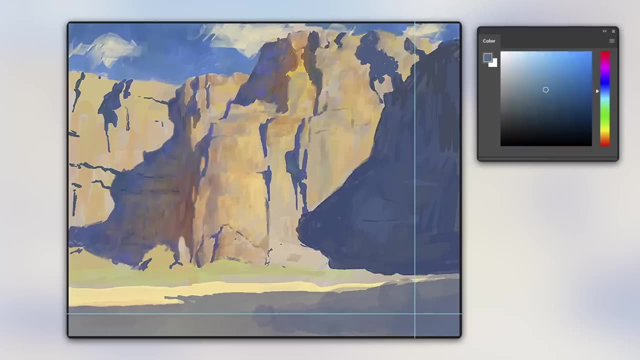 In this case, of course, also being inspired by the Edgar Payne original. Now I feel like we're putting the pain in painting. Note to self: edit that line out. So at this point I'm just working out into the rest of the painting. 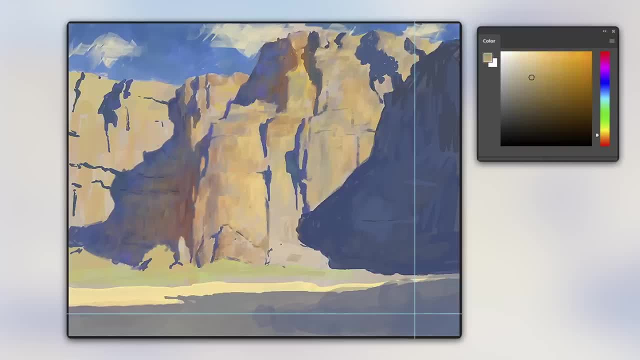 I'm tackling more of the sunlit colors here, And it might look like some of those sunlight colors are getting pretty bluish, But that's an illusion. It's actually a color shift that looks like this: Up against more saturated colors. getting grayer can look like the complement, Because that's the